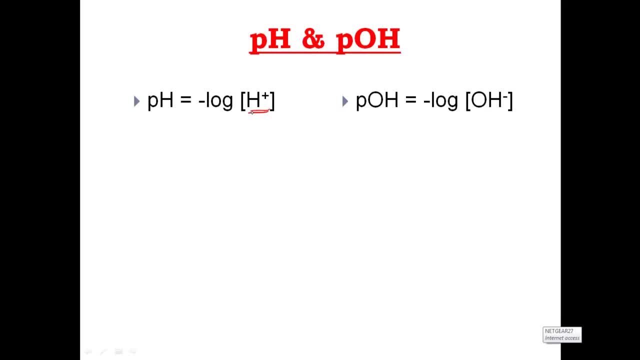 They're both calculated exactly the same way. it's just that the pH deals with the hydrogen ion and the pH deals with the hydroxide ion. Same exact way. These scales scientists use to measure the strengths of acids and bases, And you're probably pretty familiar with this. 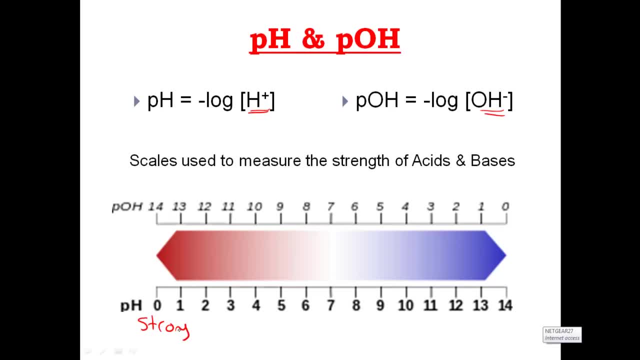 Like a strong acid is going to have a low pH. But I also want you to see the pOH scale is a little different. A fourteen on a pH pOH scale would equal a weak base, But a zero on the pOH scale would equal a strong base. 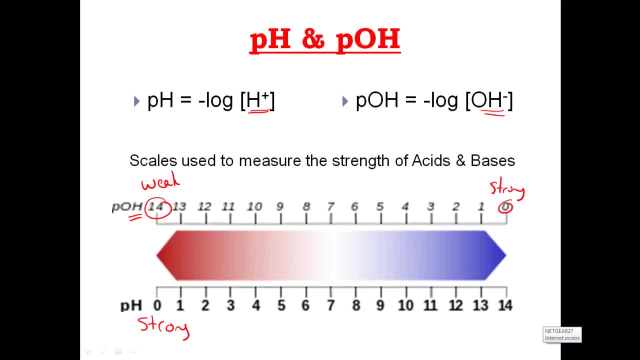 So what you're seeing here is that a base could be shown to be a strong base using a pH of 14, and a base could also be expressed as being a strong base with a pOH of zero. Likewise, a strong acid is considered as strong if it has a pH of zero. 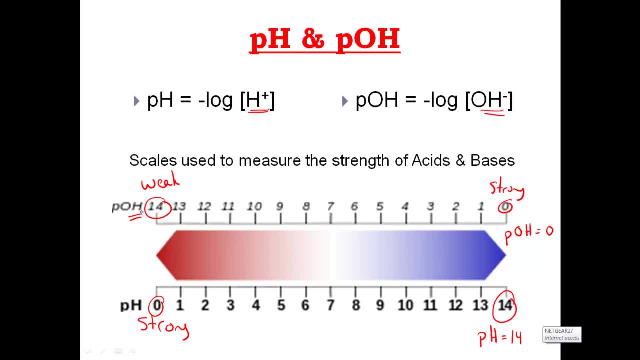 But I would have a pOH of 14.. That's right. an acid can have a pOH of zero, poh of 14, meaning it's weak as well. so what we're looking at here, guys, is different ways to measure or express the strengths of acids and bases. 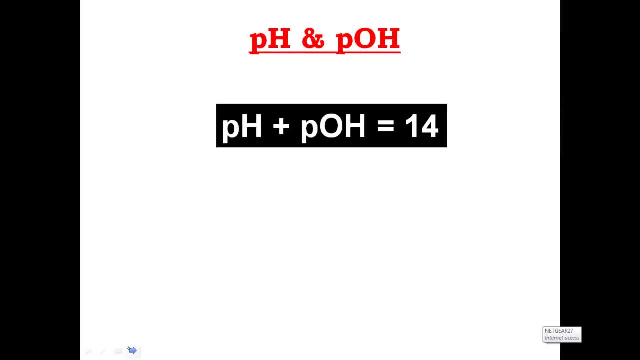 little fun fact for you: when you add up the ph and the poh, your answer will always be 14. then why don't you see that 0 plus 14 is 14, 13 plus 1 is 14. let's skip over here. 8 and 6 is 14. 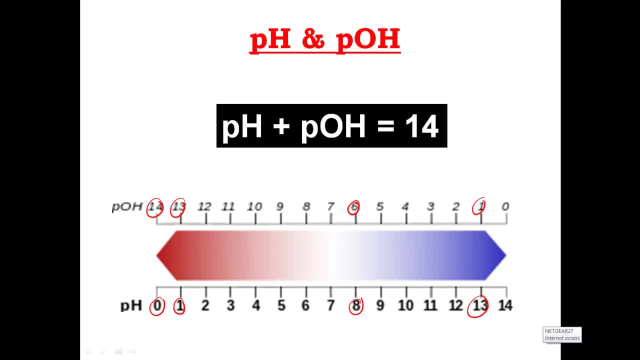 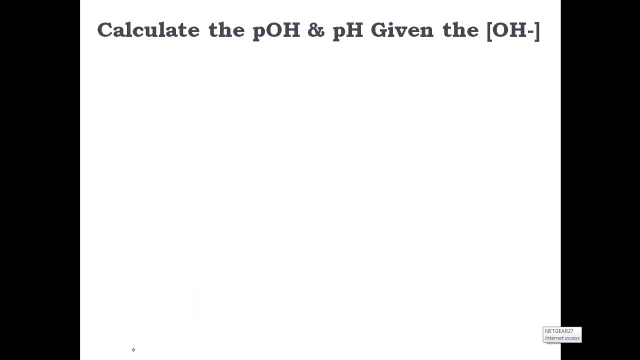 and 13 and 1, so to add up both scales, my ph and my poh, the answer is always going to be 14, and that's a useful fact for us. actually, it's a very useful fact for us. so what's going to happen here? 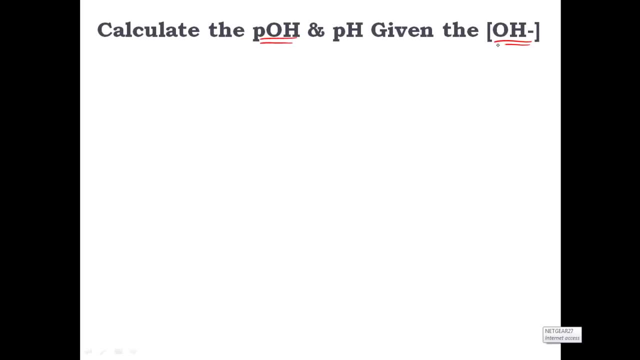 is that i want you to calculate the poh you given the hydroxide oxygen ion concentration really actually really super, duper easy. if the problem expresses the hydroxide ion concentration, the negative log, just like we solve with ph, would give me the poh. once you're given the poh, it's kind of easy actually, because the poh plus. 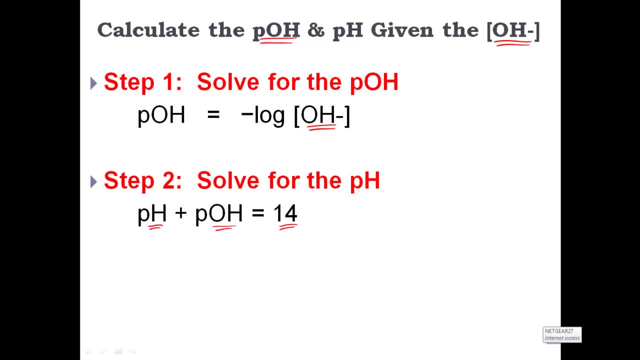 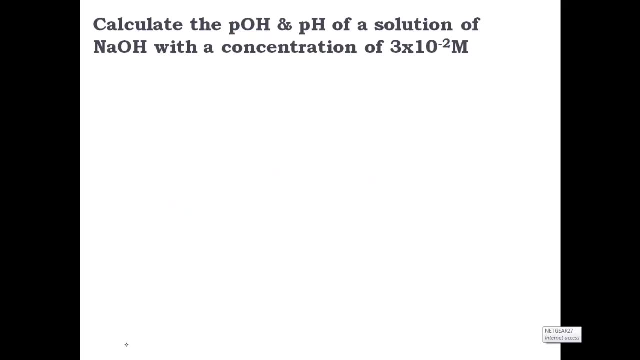 the ph is going to equal 14, man. once you know that it's an easy subtraction problem, you rearrange and say: ph equals 14 minus the poh. really, guys, really super, duper simple for us tonight here. all right, let's calculate the poh and the ph of a solution of naoh with a concentration of three. 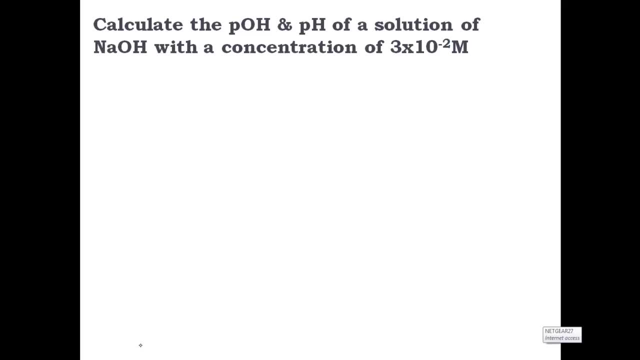 times 10 to the negative. second: all right, dudes, let's wrap our brains around this one. get a calculator out, and why don't you try to start solving this problem? step one: the p? ohb is going to be equal to the negative log of my hydroxide ion concentration, which 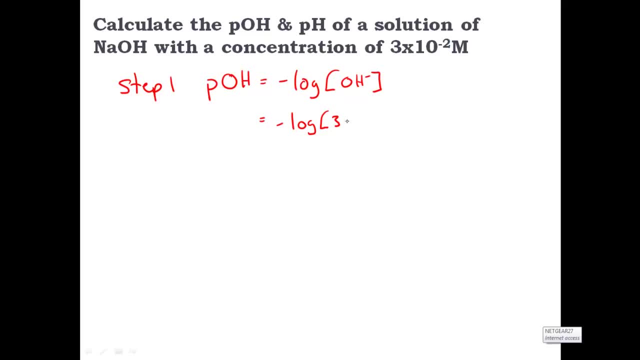 means the negative log of three times 10 to the negative second. why do you use, why'd you take two seconds to calculate that, to double-check that you're getting the same answers made me that you can use your calculators pretty good and we have a pOH of 1.5.. So on part one we find out my pOH is 1.5.. Once again, I'm just using. 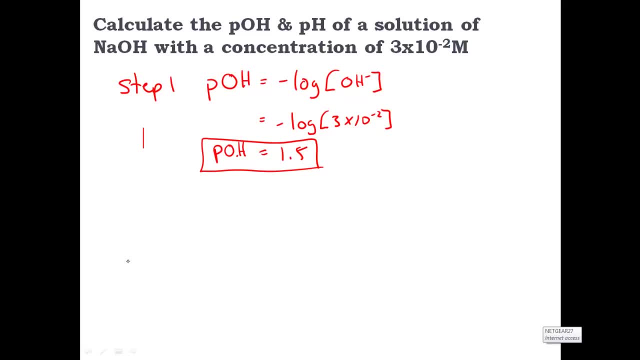 the hydrogen ion concentration In step two, we have the pH is going to be equal to 14 minus the pOH. So we have the pH is equal to 14 minus 1.5, and therefore the pH is going to be equal to 12.5.. So here's the deal, dudes. We've solved the problem. now Given you the. 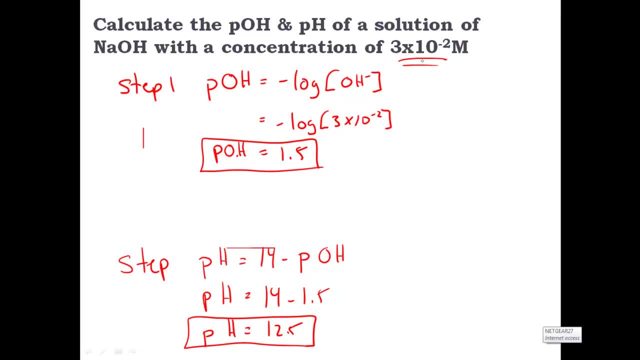 concentration of the hydroxide ion, we found a pOH. The pOH said that this is a pretty, pretty strong base If it has a pOH of 1.5, remember, a pOH of 0 indicated a really strong base. This is. 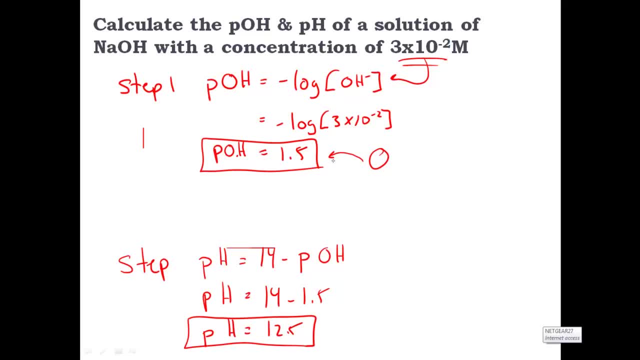 a pOH of 1.5.. Now does that make sense on our pH scale? Well, a pH scale greater than 7 is basic, and this is a 12.5 pH. So, yes, it supports the fact that with a 12.5 pH is.